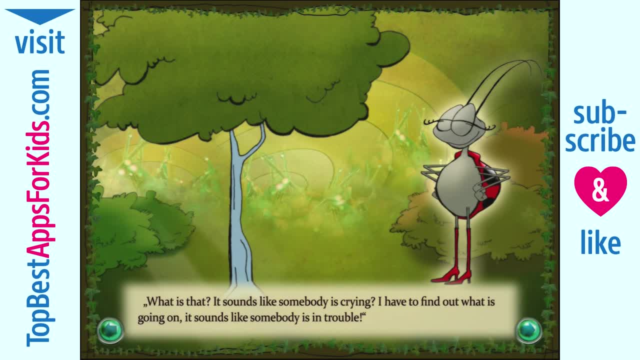 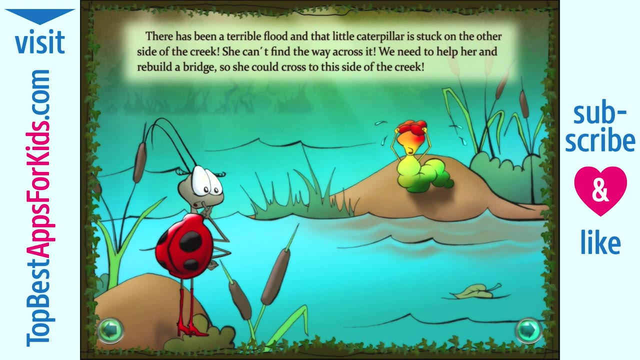 What is that? It sounds like somebody is crying. I have to find out what is going on. It sounds like somebody is in trouble. There has been a terrible flood and that little caterpillar is stuck on the other side of the creek. She can't find the way across it. We need to help her and rebuild a bridge so she could. 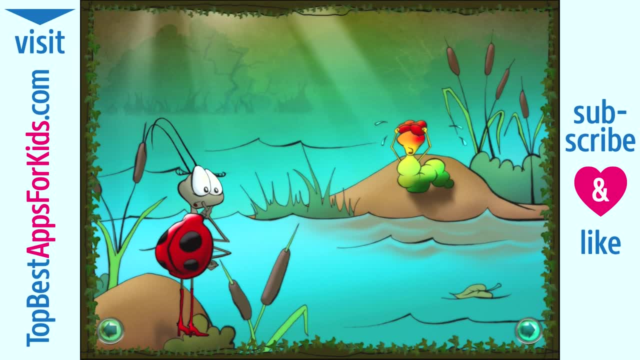 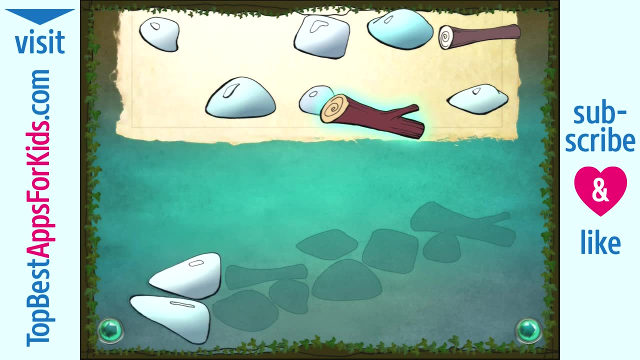 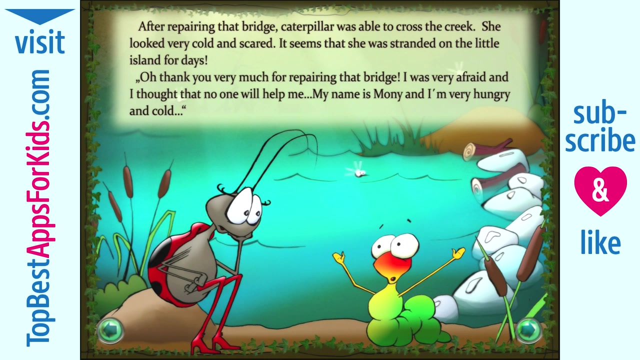 cross to this side of the creek. After repairing that bridge, Caterpillar was able to cross the creek. She looked very cold and scared. It seems that she was stranded on the little island for days. Oh, thank you very much for repairing that bridge. 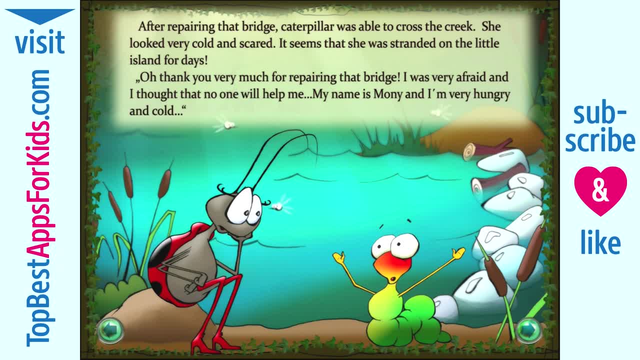 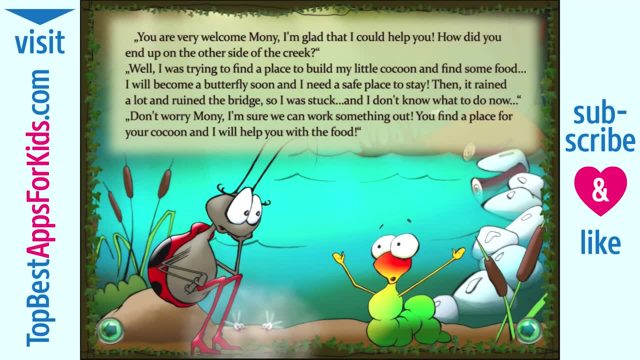 I was very afraid and I thought no one would help me. My name is Moni and I'm very hungry and cold. You are very welcome, Moni. I'm glad that I can help you. How did you end up on the other side of the creek? 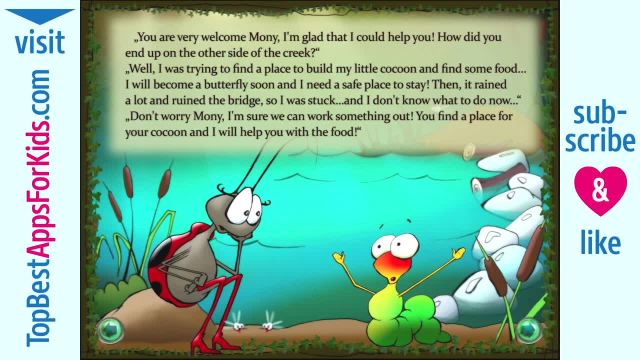 Well, I was trying to find a place to build my little cocoon and find some food. I will become a butterfly soon and I need a safe place to stay. Then it rained a lot and ruined the bridge, so I was stuck and I don't know what to do now. 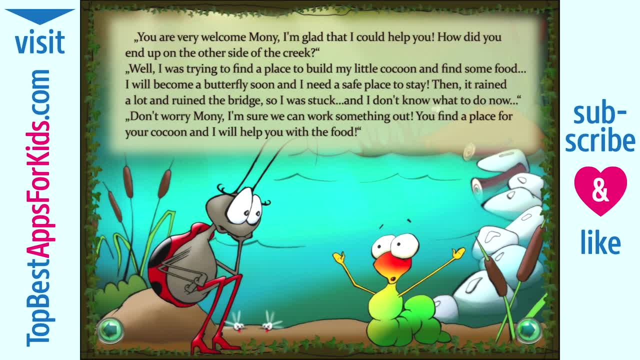 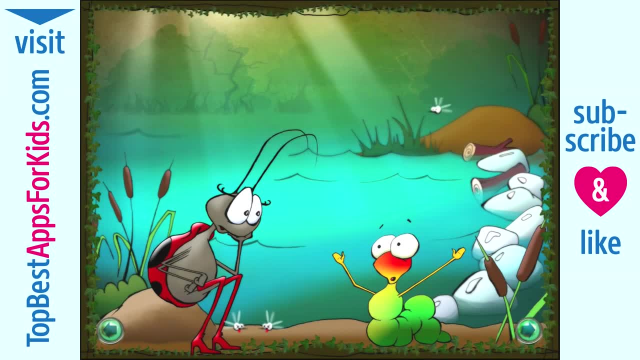 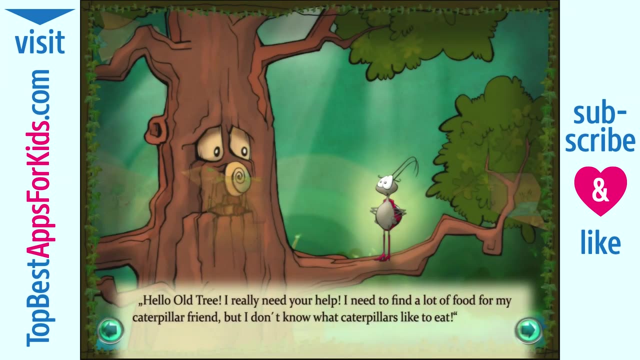 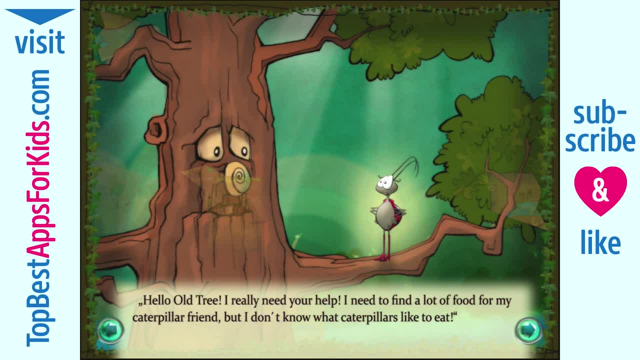 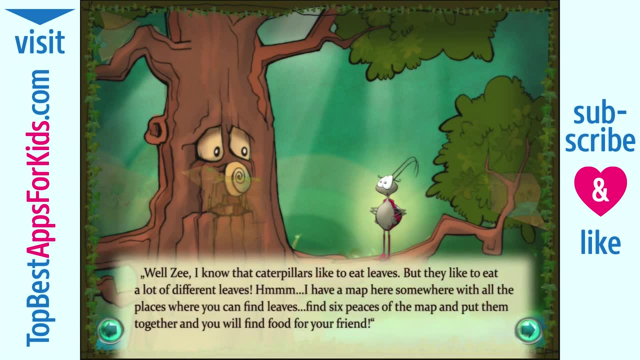 I need to find a lot of food for my caterpillar friend, but I don't know what caterpillars like to eat. Well, Ze, I know that caterpillars like to eat leaves, but they like to eat a lot of different leaves. 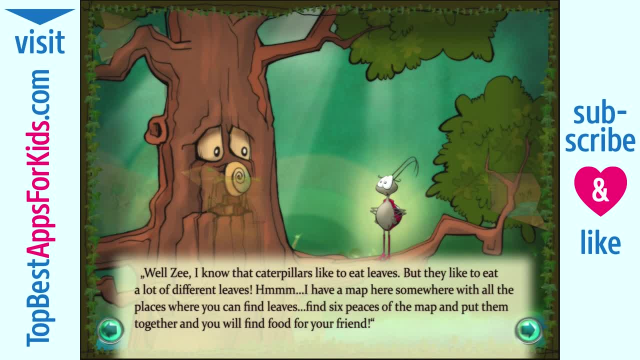 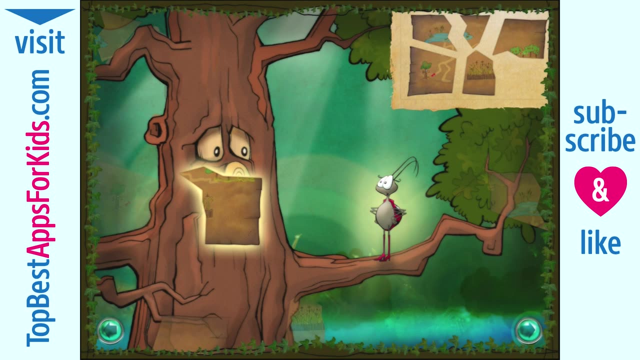 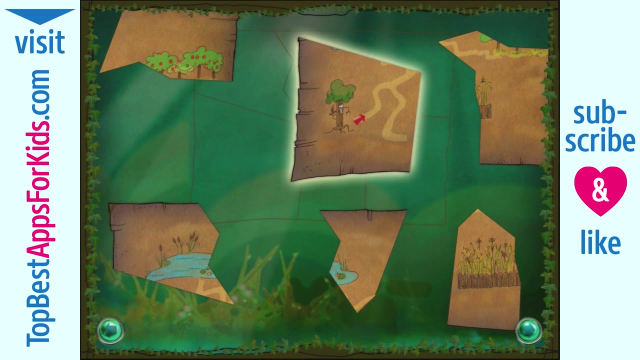 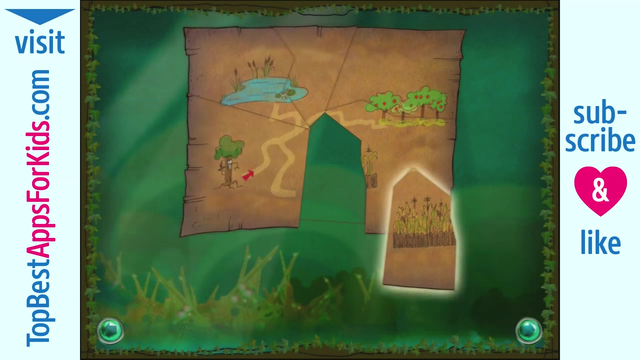 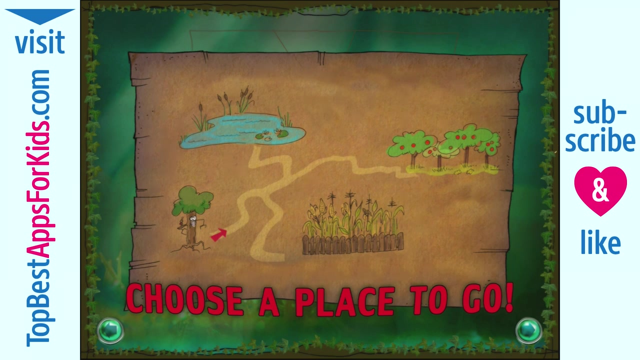 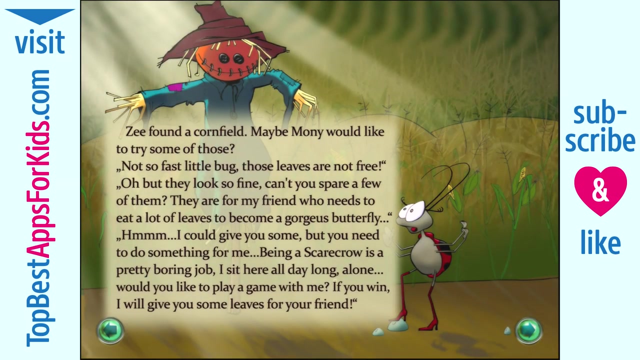 Hmm, I have a map here somewhere with all the places where you can find leaves. Find six pieces of the map and put them together and you will find food for your friend. Zee found a cornfield. Maybe Moni would like to try some of those. 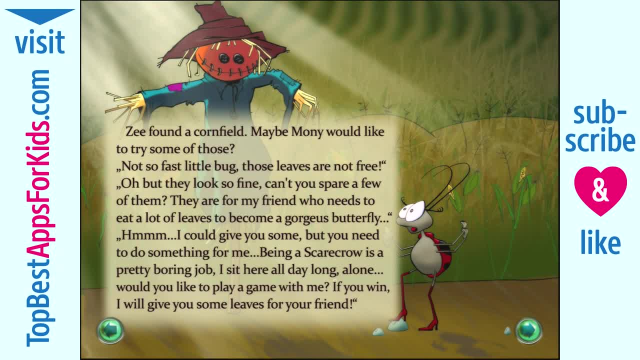 Not so fast, little bug. Those leaves are not free. Oh, but they look so fine, Can't you see? Can't you spare a few of them? They are for my friend who needs to eat a lot of leaves to become a gorgeous butterfly. Hmm, I could give you some. 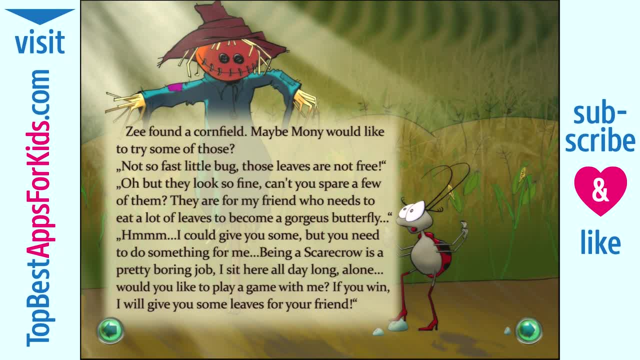 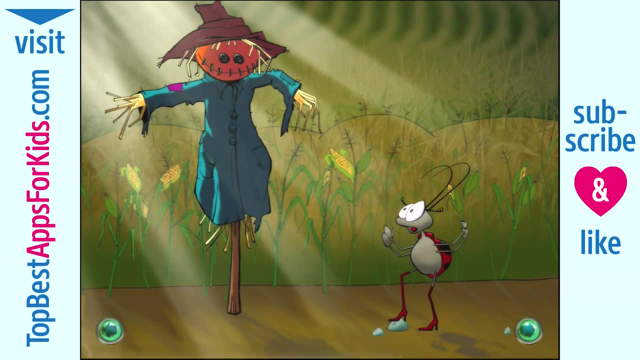 but you need to do something. for me, Being a scarecrow is a pretty boring job. I sit here all day long alone. Would you like to play a game with me? If you win, I will give you some leaves for your friend. Hey, do you know a game called? 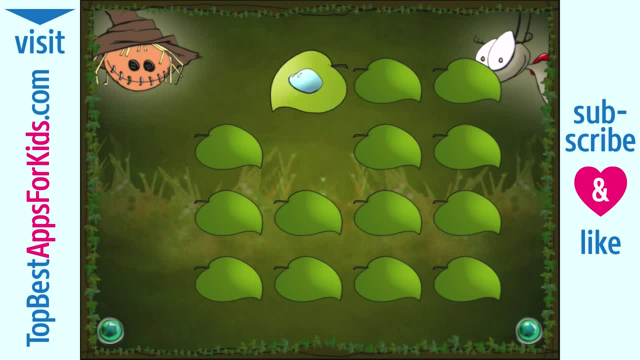 What appears to order. A game called What appears to order is A game called What appears to order is a detail which can't be named, And now is exactly the meaning of what it is: Self play. Take a look at the name or change child's name. 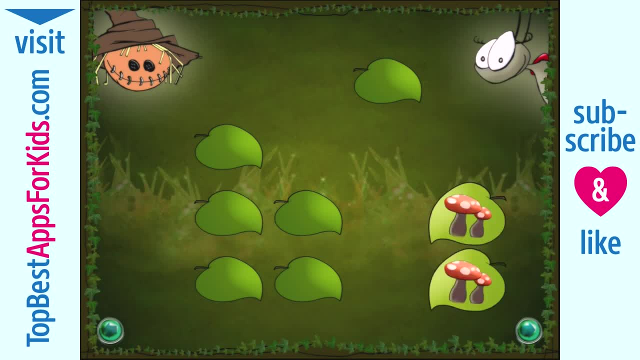 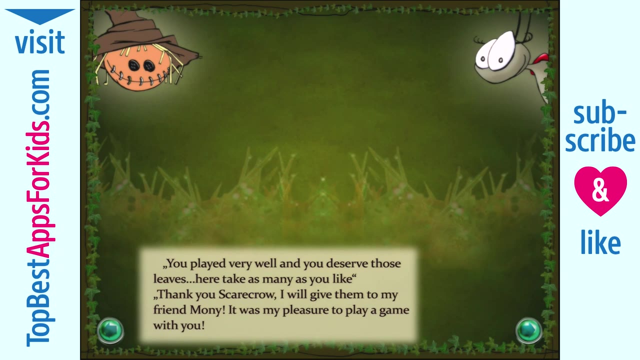 A sample isского, A set isboys And a ED. You can choose three presentations: A three-, dimensional, A four dimension, Colonial, R unearltonarn. You played very well and you deserve those leaves Here. take as many as you like. 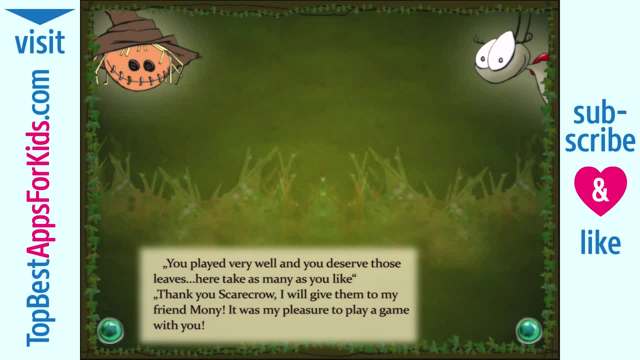 Thank you, Scarecrow. I will give them to my friend Moni. It was my pleasure to play a game with you.